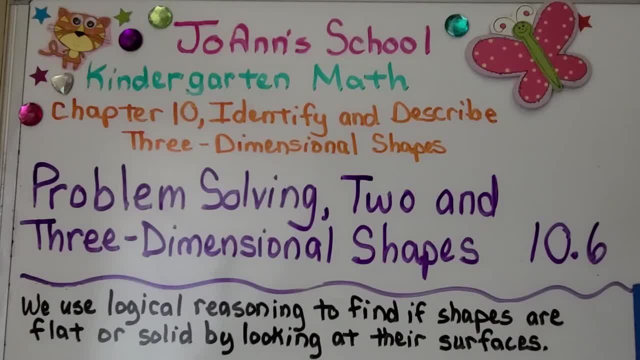 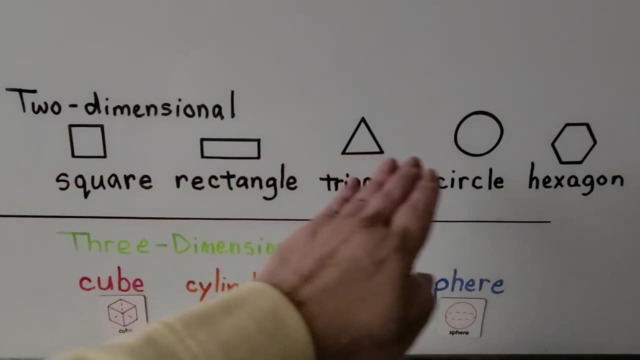 Lesson 10.6. Problem Solving Two- and Three-Dimensional Shapes. We use logical reasoning to find if shapes are flat or solid by looking at their surfaces. Two-dimensional shapes are flat. They're flat shapes: A square, rectangle, triangle, circle, hexagon. These are two-dimensional shapes. 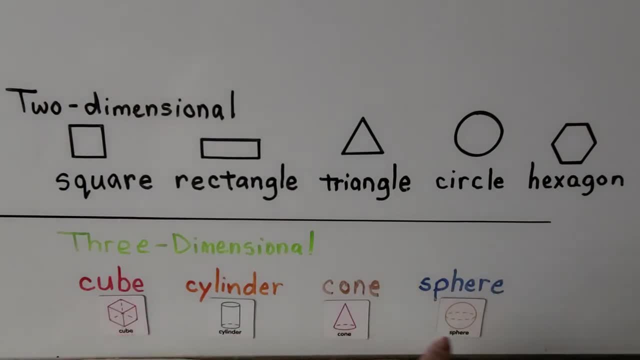 Three-dimensional shapes are solid shapes. They take up space. The surfaces of three-dimensional solid shapes are flat or curved, But the whole thing is flat. The whole shape takes up space. Solid shapes have surfaces that look like flat surfaces And some solids, like a sphere has no flat surface. 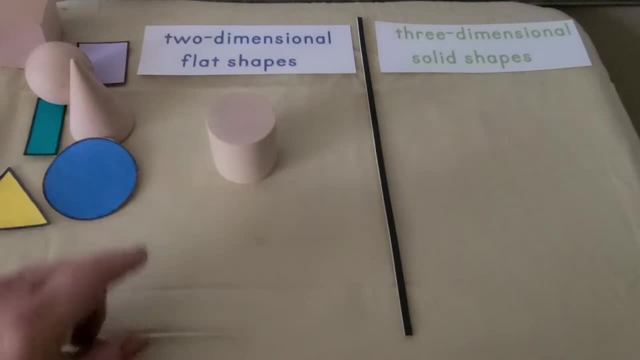 A solid shape can have a shadow. See its shadow. A flat shape doesn't have a shadow, It's just flat 庇 OO. We can sort all of these shapes into sets of two-dimensional flat shapes and three-dimensional solid shapes. We can look for a shadow, we can look for curves or we can see if it takes up. 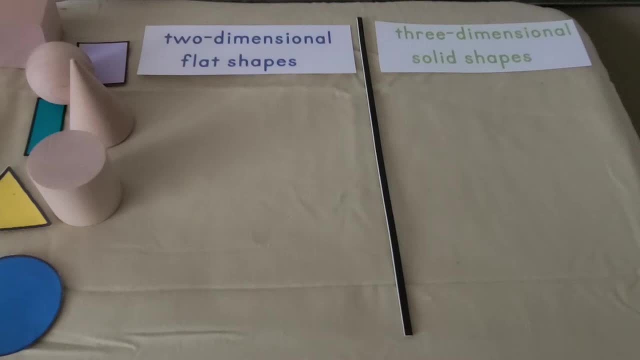 space, or it's a three-dimensional solid shape. We can see this shape and something else. This is what we call an innovation. We do this for labor, But our task is to look for them continuously takes up space. It's not flat. It has two flat surfaces and a curved surface. This 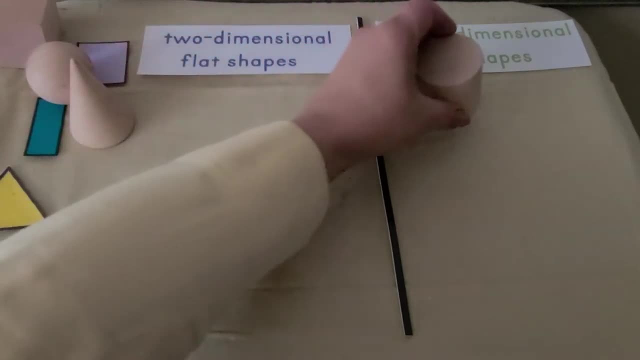 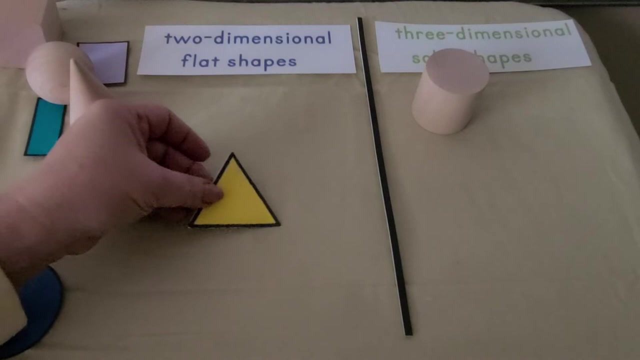 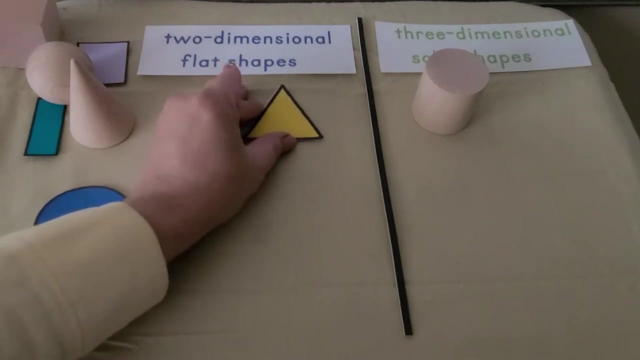 is a cylinder. That's a three-dimensional solid shape. This is a flat shape. That's a triangle. That's a two-dimensional flat shape. This is a circle. This is a flat shape. This is a two-dimensional flat shape. This shape has a shadow. It takes up space. It. 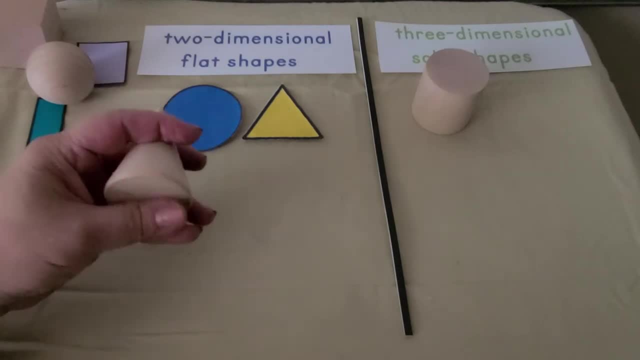 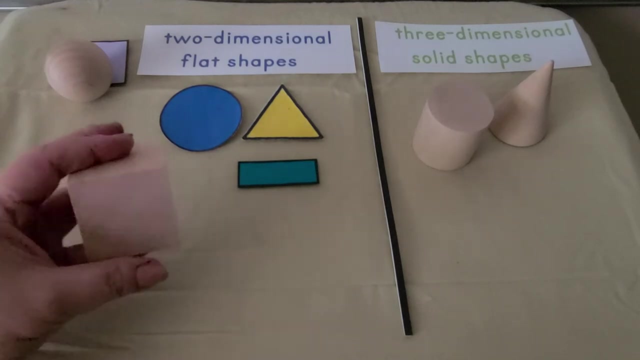 has a curved surface and it has a flat surface. This is a cone. That's a three-dimensional solid shape. Here's a flat shape That's a rectangle. It has four sides that are straight. It has four square corners. That's a two-dimensional flat shape. This has six flat sides that are 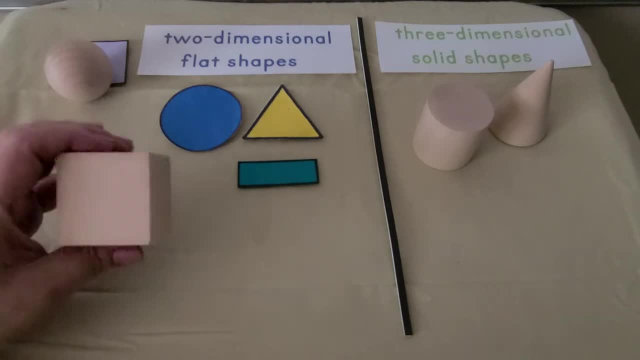 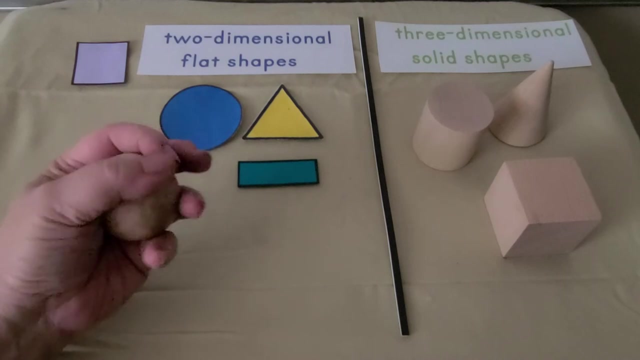 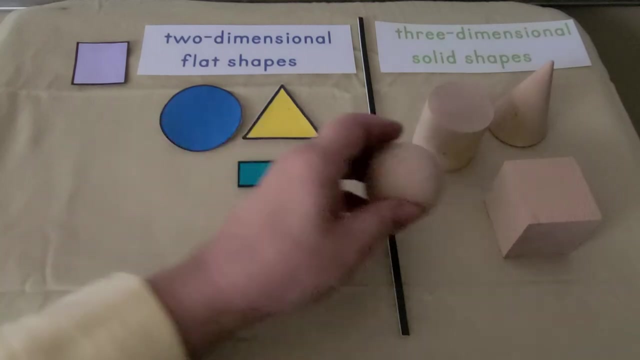 shaped like squares. This is a solid. This is a cube And this has no flat surfaces. We can see it has a shadow and it takes up space. It's got a curved surface. This is a solid shape. This is a sphere. This is a. 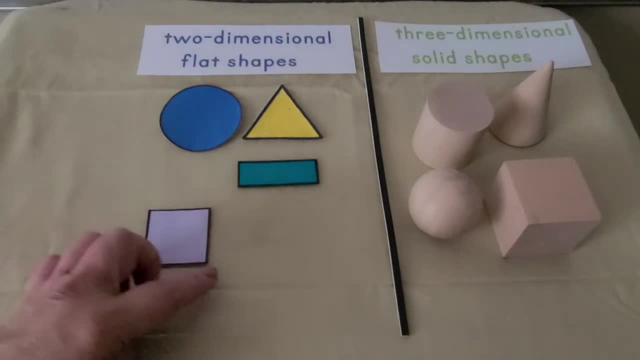 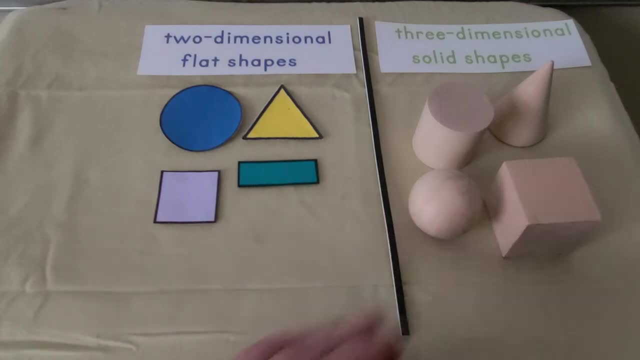 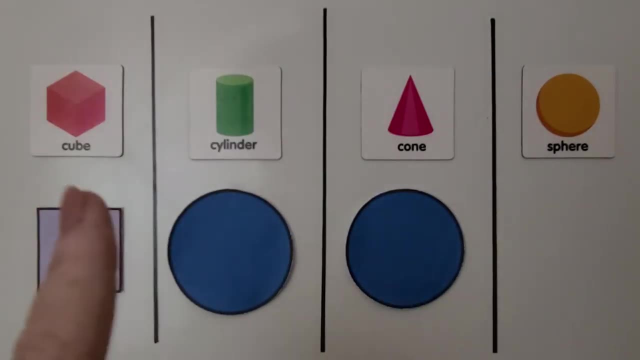 The flat shapes are two-dimensional. The solid shapes are three-dimensional. A cube is still a solid shape. has six flat square surfaces that are all the same size. A cylinder is still a square shape. is a solid shapehod. A cylinder is当 sizes. 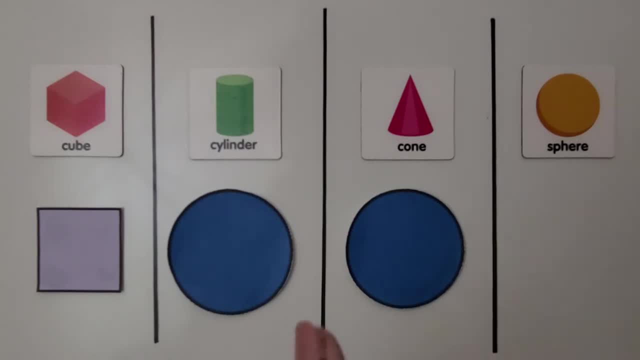 A cylinder wheel vosstad was laid. A cylinder wheel vosstad was laid. solid shape that has two flat surfaces and one curved surface. Its surfaces- two flat surfaces- can be shaped like circles. A cone is a solid shape that has a flat. 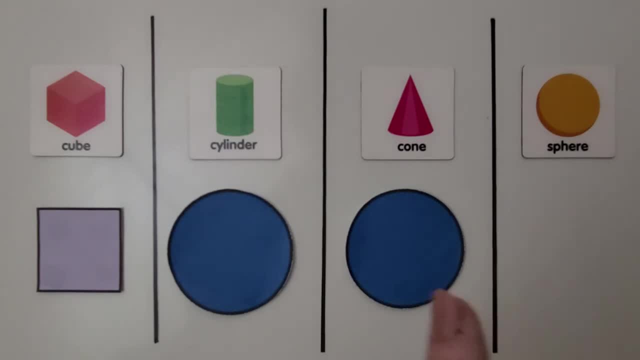 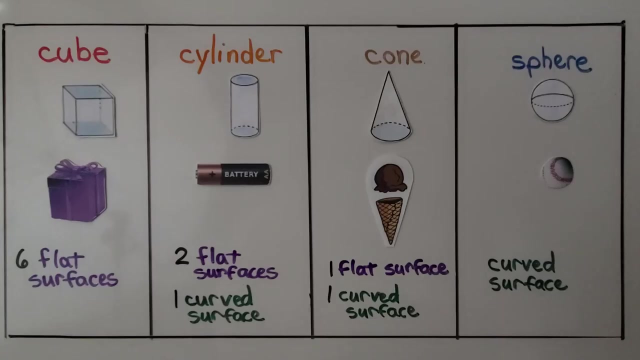 surface and a curved surface, and its flat surface could be shaped like a circle. A sphere is a solid shape that has no flat surfaces. It's shaped like a baseball. There are things all around us that are shaped like solid figures. A birthday present box could be shaped like a cube. a battery is shaped like a.